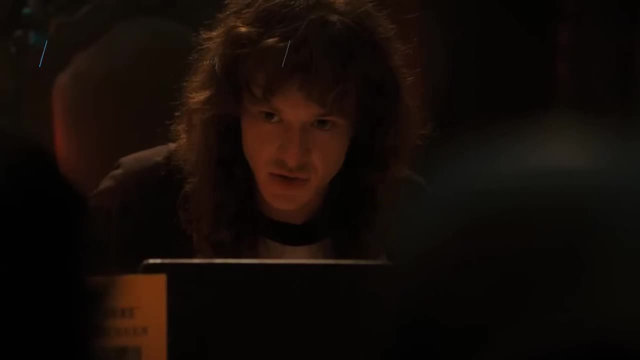 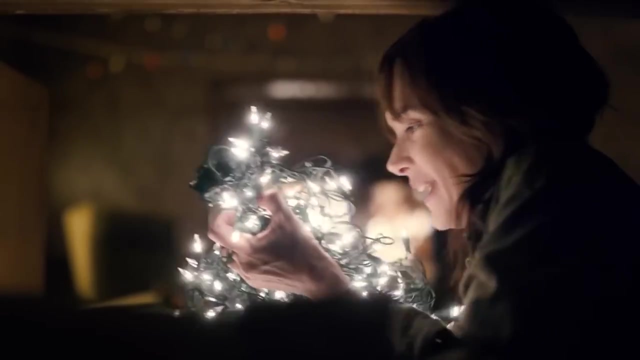 its purse strings. one show that the platform has funneled endless money into is the hit supernatural sci-fi series Stranger Things. Since the show's $6 million per episode freshman's season, Netflix has gradually increased its budget while continuing to ramp up the killer. 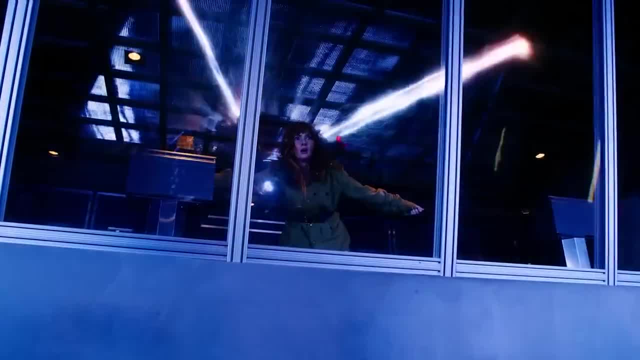 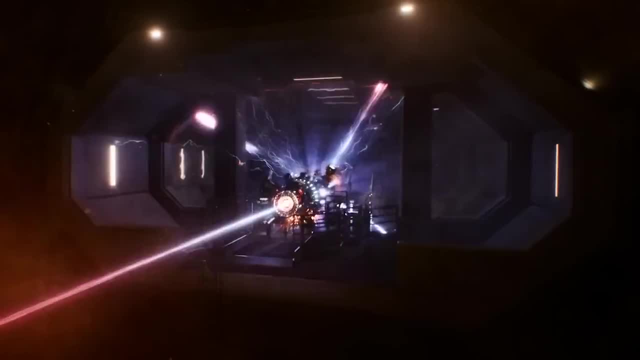 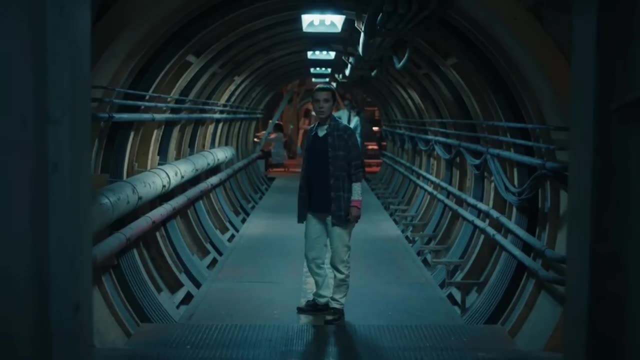 computer-generated and practical effects. Not only that, but by 2018, several of the show's cast were taking home paychecks of around $250K to $350K per episode. It's estimated that the price tag for the fourth season came in at around $30 million per episode, According to Netflix. 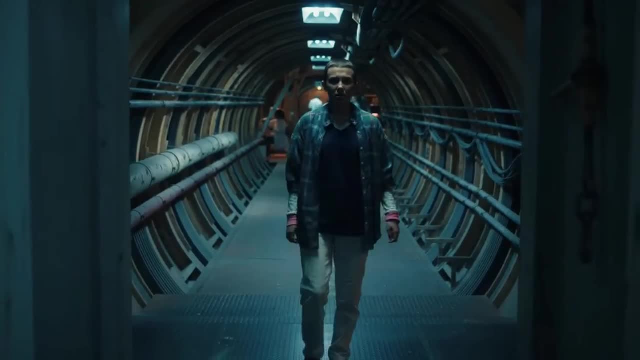 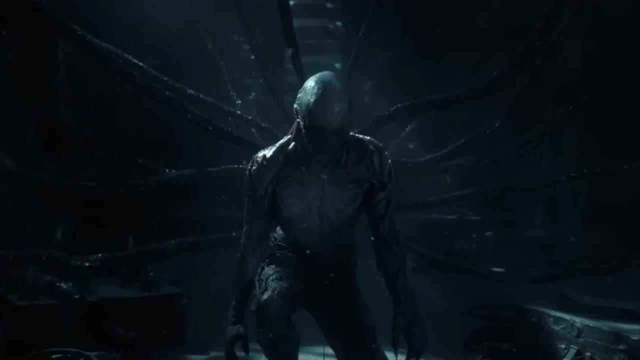 executive, Ted Sarandos. a hefty chunk of season four spending increase can be attributed to COVID which, between the need for extra protocols and production shutdowns, hit the budget hard. Still, it was money well spent. The show features some of the most beautiful CGI out there. 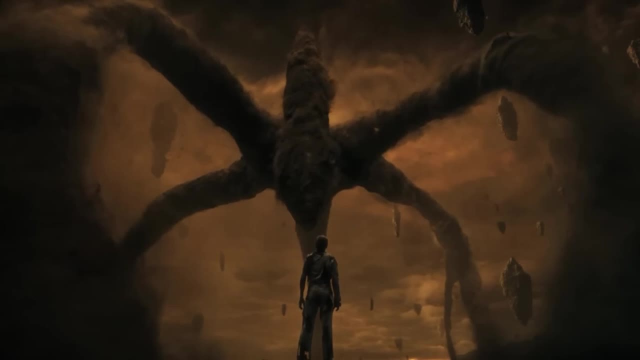 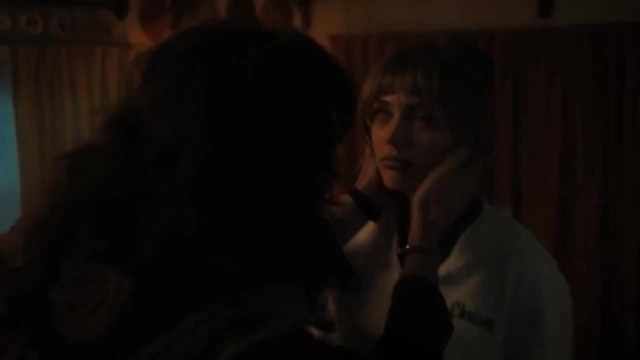 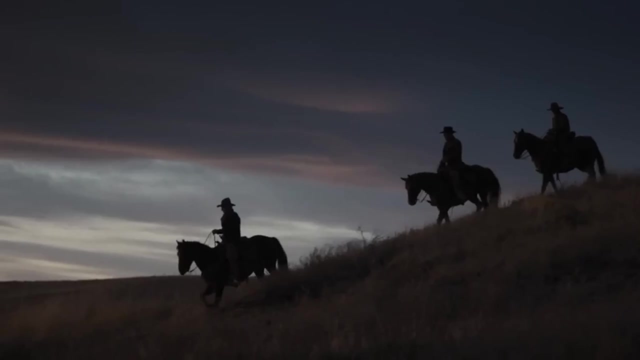 and is a testament to the truly cinematic quality a well-executed streaming series can have This attention to detail, even earned Stranger Things the Emmy for Best Prosthetic Makeup in 2022.. The second prequel to Taylor Sheridan's hit series Yellowstone 1923, follows the Dutton family during 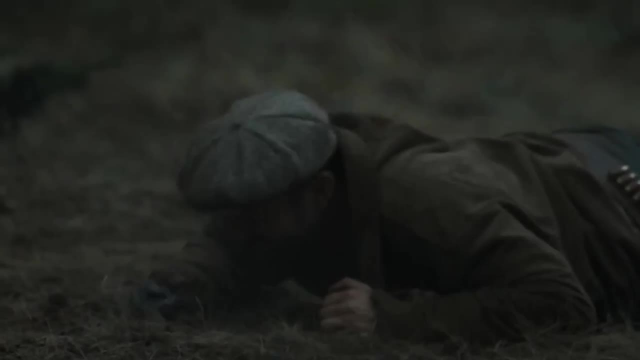 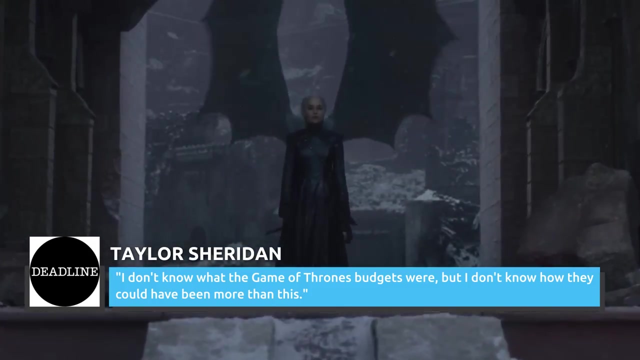 the Great Depression. Comparing his latest show to Lawrence of Arabia in terms of scale, Sheridan told Deadline: I don't know what the Game of Thrones budgets were, but I don't know how they could have been more than this. One of the show's big-ticket items is its cast, an ensemble led by Hollywood legends. 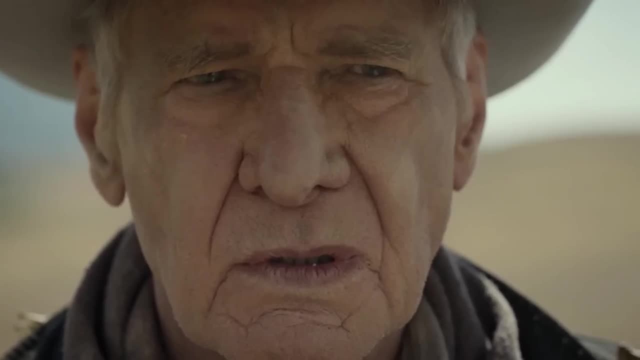 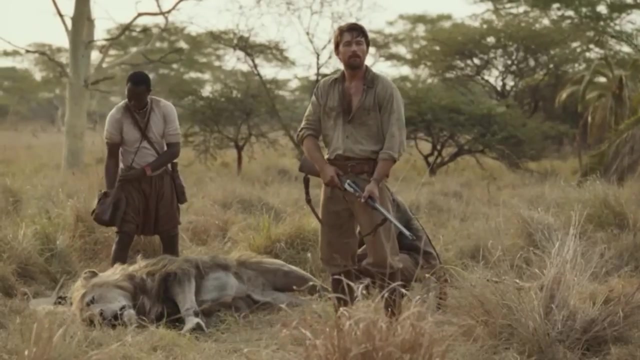 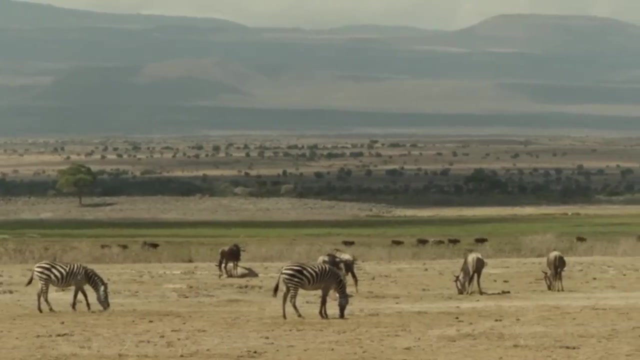 Helen Mirren and Harrison Ford. But this is just the beginning. To create the sense of life on a Montana ranch, the series uses thousands of real cattle and sheep and much of 1923 was filmed in, including Malta, Tanzania, Kenya and South Africa. Filming during the pandemic also meant. 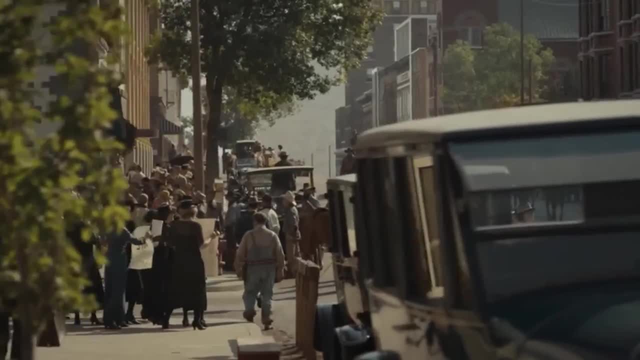 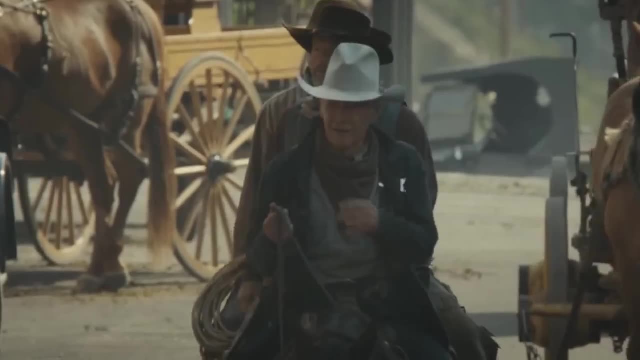 that COVID protocols upped the budget even further. Then, of course, you've got the added cost of a historical series. It's no mean feat to build in dress sets for a show set 100 years in the past. The grand total for this gorgeously rendered drama comes in at around $30 million. 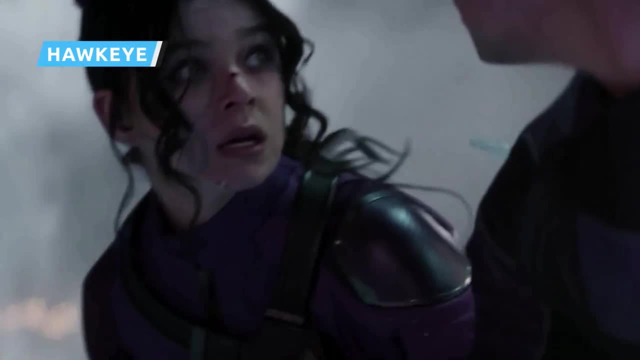 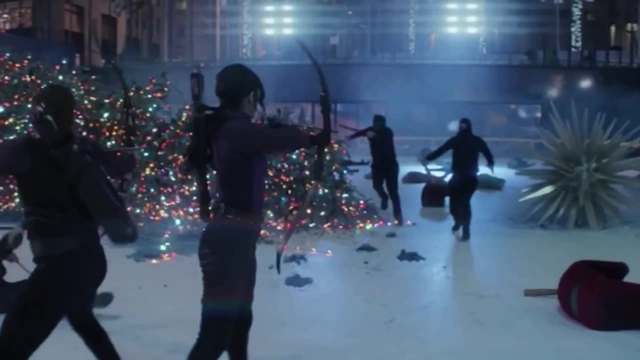 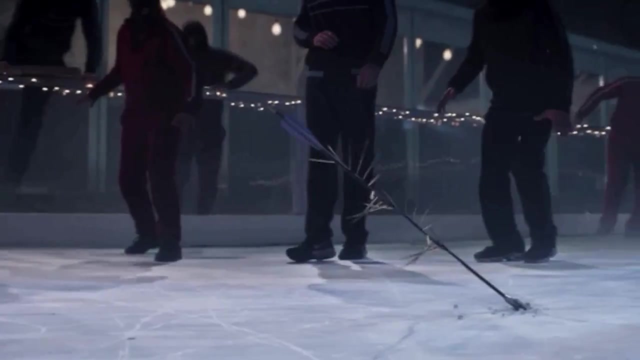 per episode. It's time, All right, Good, Let's give them hell. The MCU Disney Plus series Hawkeye racked up a $150 million price tag during its six-episode run, which comes out at around $25 million per episode. For the sake of comparison, Captain Marvel, one of Marvel's theatrical releases, boasted a budget of around $152 million. As with many other big-budget TV shows, one of Hawkeye's major costs was its star power, Jeremy Renner, who reprises his role as the titular Avenger. 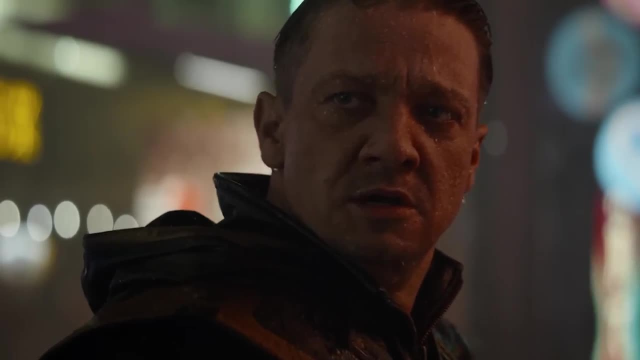 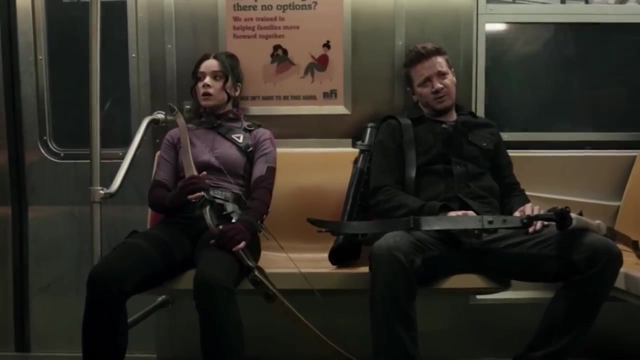 is one of the higher-paid actors in the Marvel Universe, While his salary for the series isn't widely known, Parade reported that the actor made $50 million for Avengers Endgame and likely took home a similar paycheck for Hawkeye, As the series was primarily filmed in New York City, Georgia and Ontario. 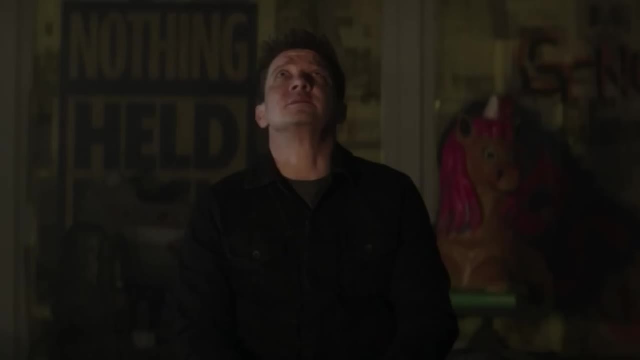 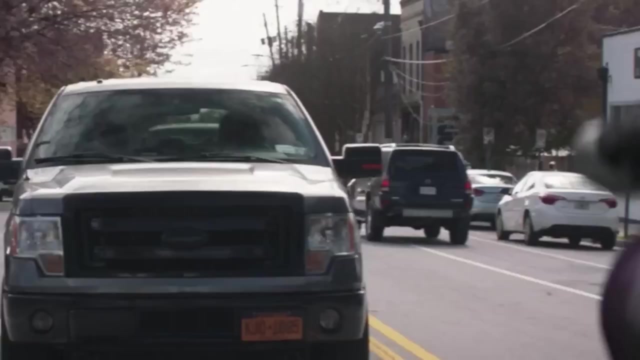 they weren't exactly dropping much of the budget on hauling an entire casting crew from one exotic location to the next. However, as is the case with many MCU shows and movies, Hawkeye will have required a significant amount of CGI, which always ramps up the budget. Judging by 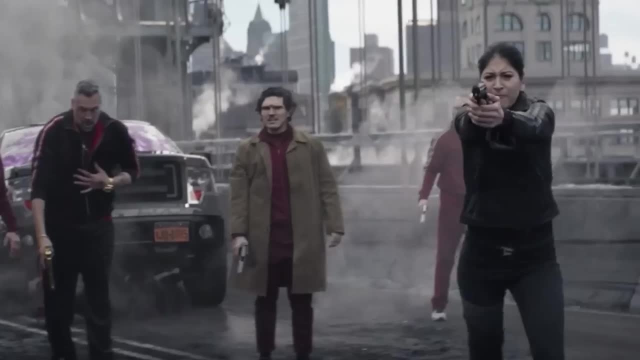 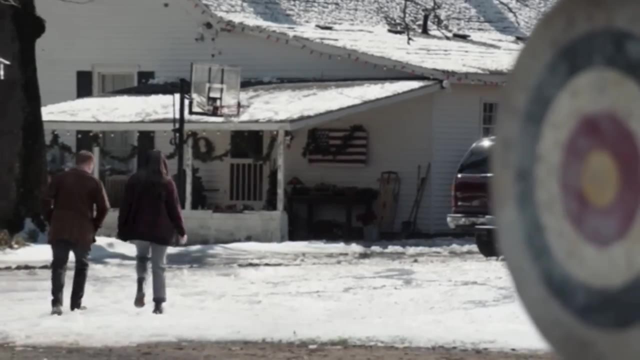 the controversy stemming from the disappointing effects in Episode III, however, as well as greater complaints about pay and working conditions from Marvel VFX teams, it seems that this is one area in which the franchise shouldn't be cutting costs, As the first Marvel series to be released. 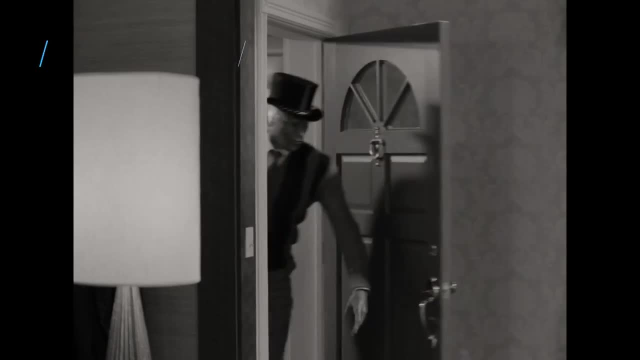 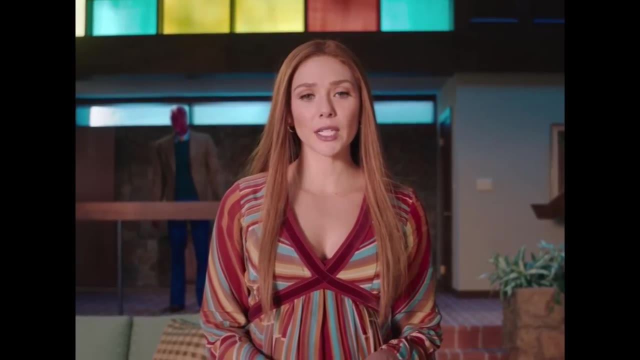 on Disney+ and the first of the MCU's Phase 4, WandaVision, was a much-hyped and well-received entry into the Marvel canon. Like the comics themselves, the MCU keeps things fresh by serving up a variety of genres and storytelling styles, and WandaVision is one of the most. popular Marvel mainstays in the franchise. As the Marvel franchise continues to grow, the Marvel franchise is in the process of growing into the next-generation Marvel franchise. As the Marvel franchise continues to grow, the Marvel franchise is in the process of growing into the next-generation. 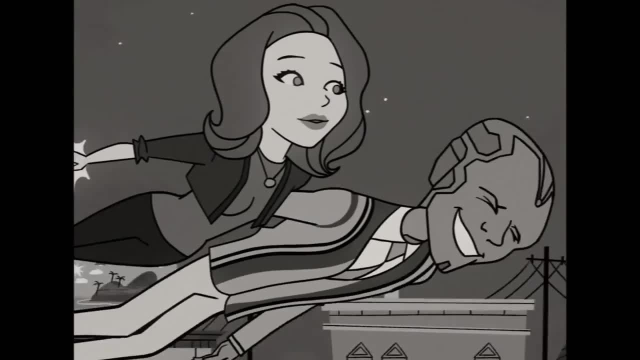 Marvel franchise. As the Marvel franchise continues to grow, the Marvel franchise continues to grow, and WandaVision is a stunning example of this. Starring Elizabeth Olsen as Wanda Maximoff and Paul Bettany as Vision. the series finds the pair trapped in a strange alternate reality. 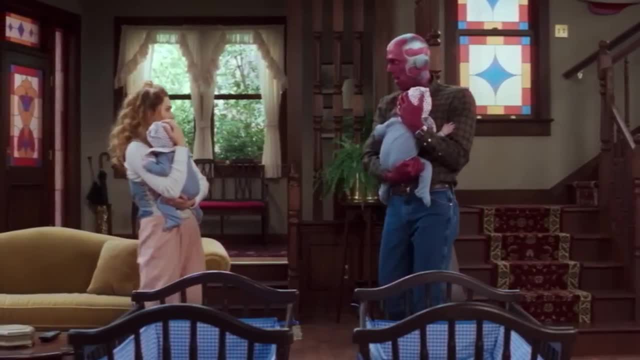 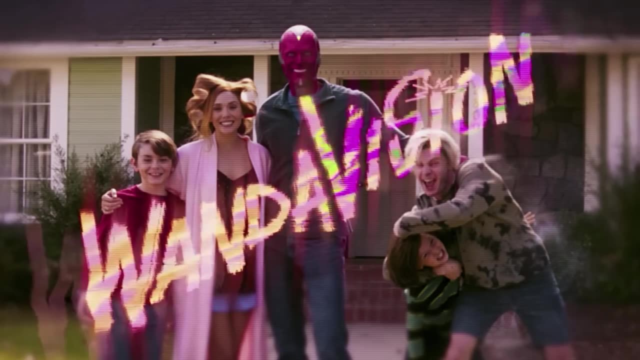 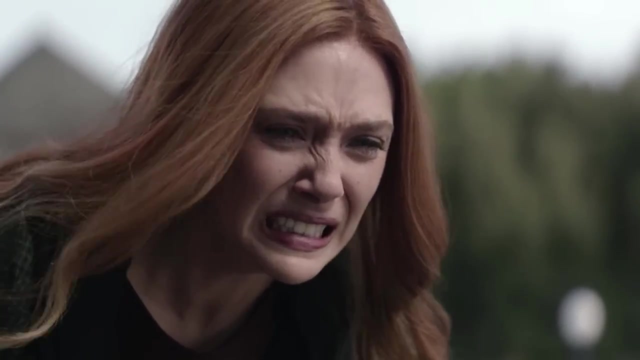 that looks and feels like a laugh-track sitcom. As the episodes progress, the pair transitions from one decade to the next, traveling through sets inspired by some of the 20th century's most beloved TV shows. Like other Marvel shows, WandaVision was given a generous budget of 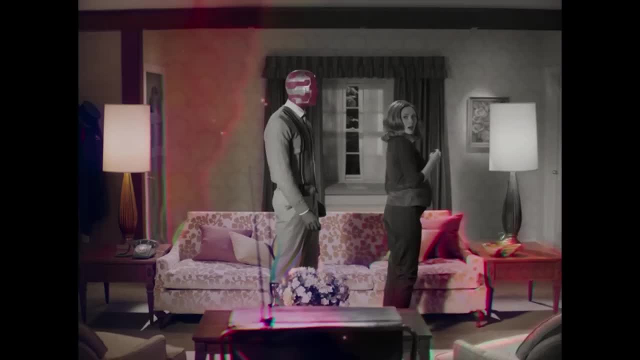 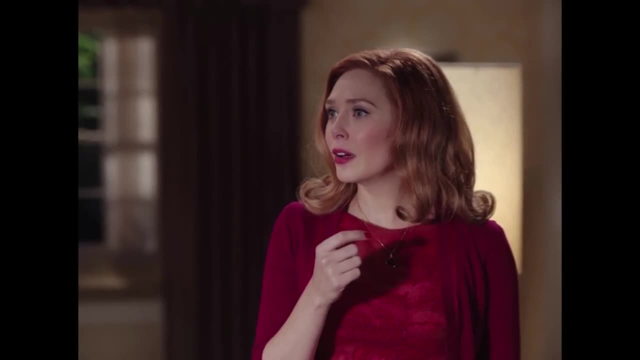 about $25 million per episode, and it shows, Besides the lead duo's inevitably impressive earnings. the show featured 400 shots of VFX created by a team of 100 or so compositors. The sequence in which Vision flies around Westview, for example, took months to produce. 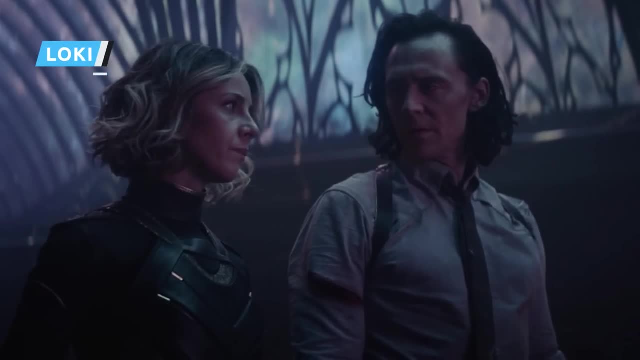 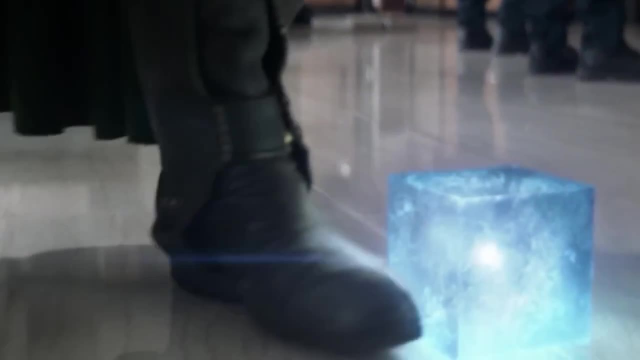 and effects like that don't come cheap. Yet another entry in Marvel's Disney Plus lineup. Loki finds the God of Mischief joining the Time Variance Authority to repair the damage to the timeline caused when he swiped the Tesseract in Avengers. 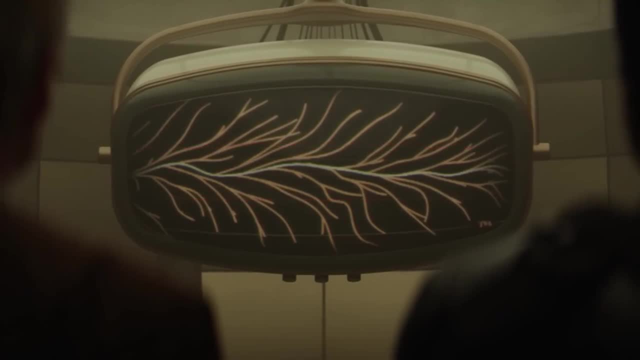 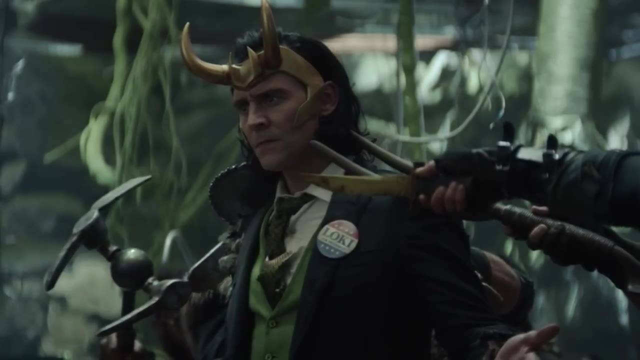 Endgame. This wickedly fun time-travel twister is one of the best recent offerings from Marvel Studios. Although with a budget of about $25 million per episode, it certainly wasn't cheap. As you've probably guessed, Loki stars Tom Hiddleston as the MCU's favorite trickster. 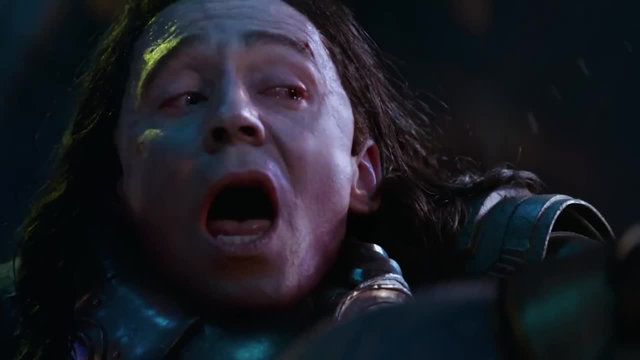 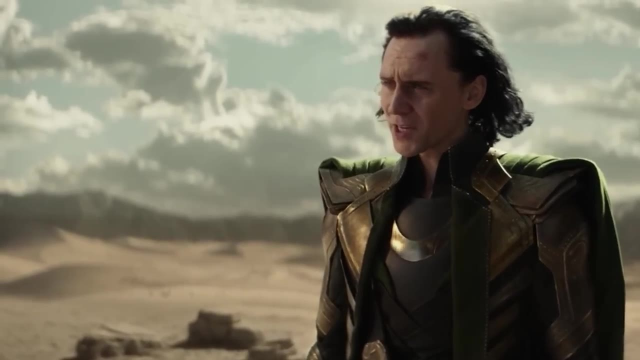 And considering he was reported to have been paid $8 million for his very brief role in Avengers Infinity War, it's safe to say that a decent chunk of the show's budget went toward his paycheck. All that money, at least, seems to have paid off. however, Many fans and critics agreed that the series felt more like a film than a TV show, and the first season was nominated for six Emmys, including one for costumes and another for outstanding production design. Perhaps unsurprisingly, The Falcon and the Winter Soldier enjoyed a comparable budget to WandaVision and Loki, at around $25 million per episode. The show takes place a few months. 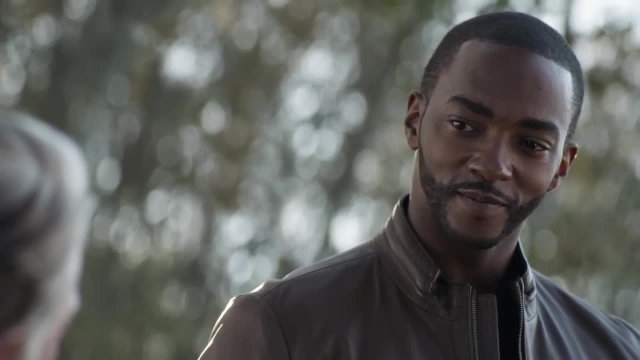 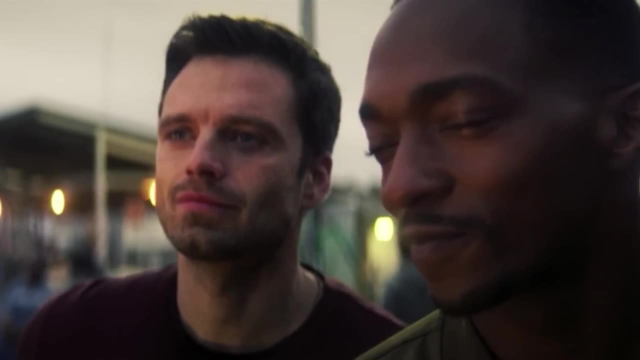 after Avengers Endgame, which ended with Sam Wilson taking up Captain America's shield, Anthony Mackie and Sebastian Stan reprise their roles from the movies, and the show didn't exactly skimp on it. not only that, but The Falcon and the Winter Soldier was partly filmed in the Czech Republic. 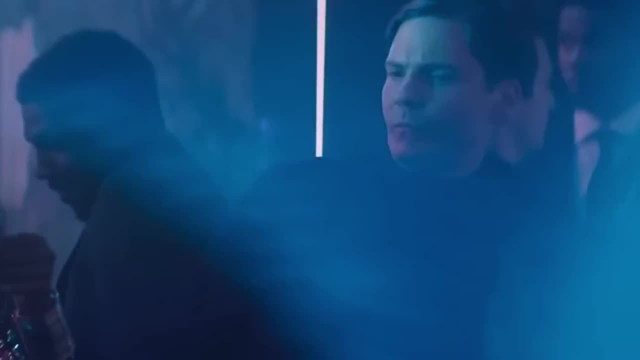 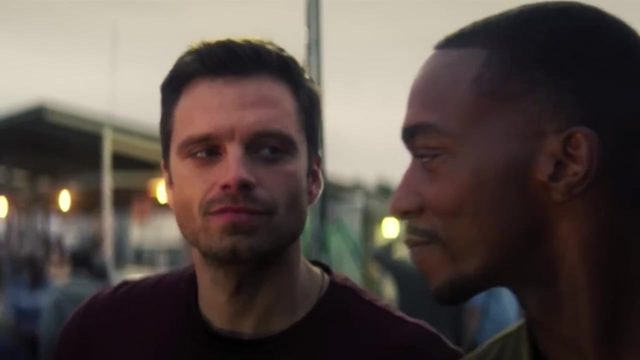 Hence the COVID outbreak of 2020 completely halted production for several months, too likely adding a significant number to the show's final cost. While some critics felt the show's early pacing could have been better, overall it drew praise for its social commentary and the chemistry between its leading actors. 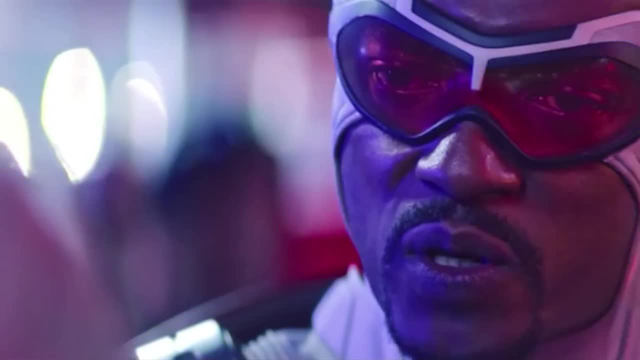 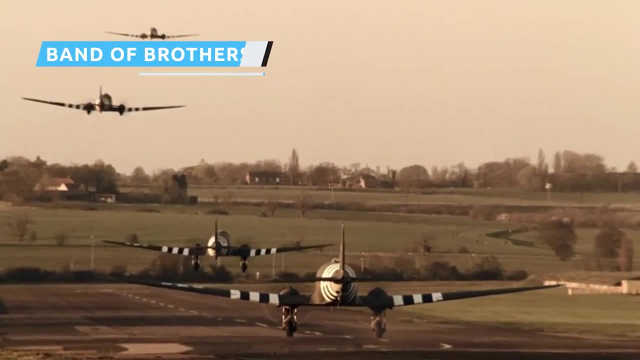 Falcon and the Winter Soldier's budget is clearly well spent too, making it an enjoyable series overall, even if it isn't the strongest limited series Marvel has ever produced. These days, a blockbuster movie budget is hardly a rarity in the world of TV production. 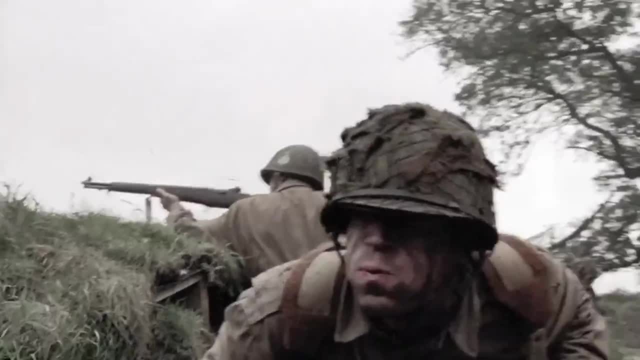 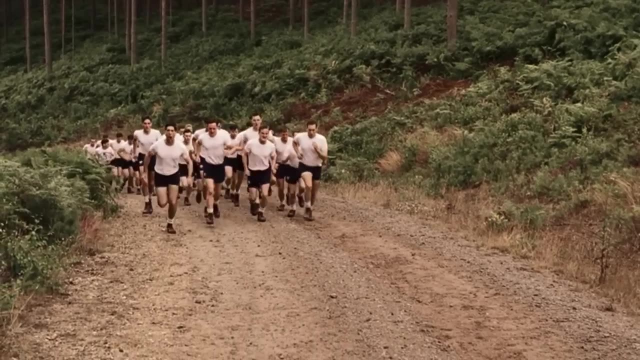 In 2001,. however, it was practically unheard of. Produced by Steven Spielberg and Tom Hanks, Band of Brothers was the most expensive television production to date, with a budget of $125 million, which would be closer to $200 million today. 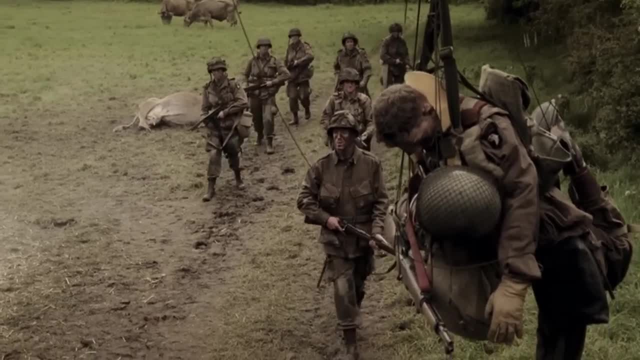 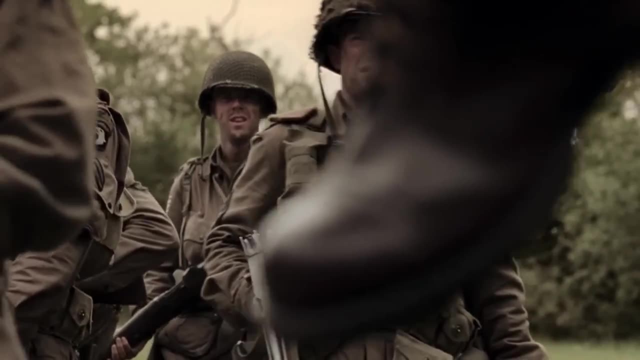 The 10-part miniseries follows Easy Company, a group of World War II paratroopers from the 101st Airborne Division, From training through their deployment on D-Day and ultimately to the very end of the war. a large portion of Band of Brothers' budget went. 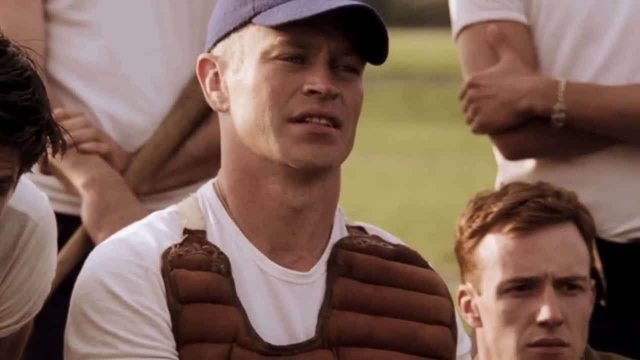 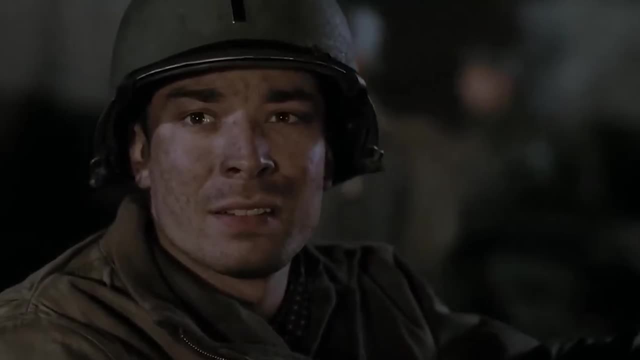 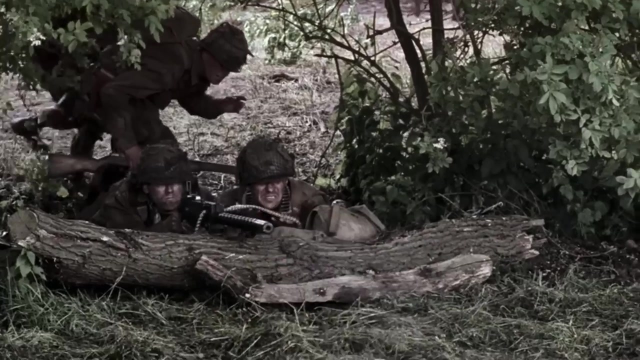 to support the massive ensemble cast, many of whom were relatively unknown at the time of filming but have since gone on to become famous faces today. In the interest of depicting the war as accurately as possible, the filmmakers and cast consulted many of Easy Company's surviving veterans, invested in authentic uniforms and 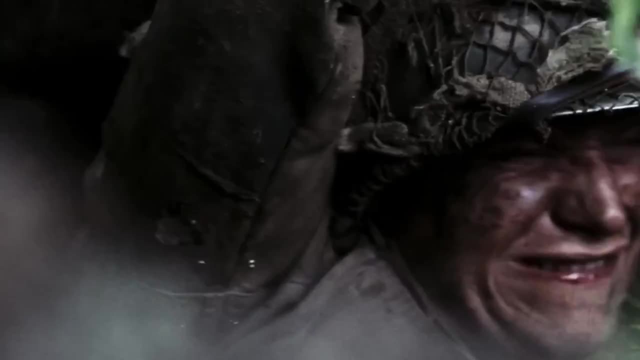 equipment and poured plenty of their time and effort into the film. The film was a great success and many of Easy Company's veterans were able to make their mark on the world of television. The effort paid off, with many World War II veterans and history experts alike. 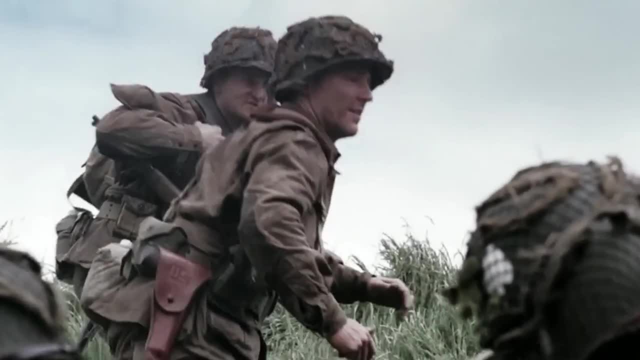 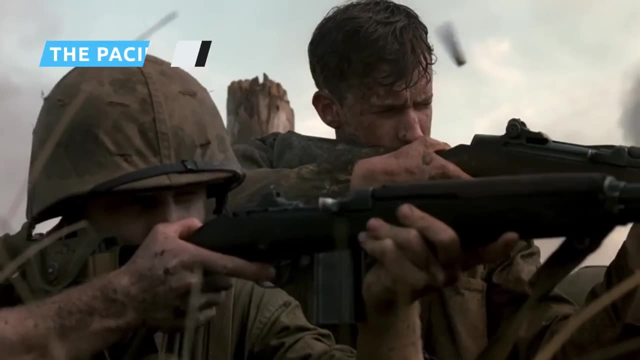 agreeing that the series presented one of the most accurate portrayals a World War film ever produced. The Pacific is a 2010 production that serves as a companion piece to Band of Brothers. Much like its older sibling, The Pacific became the most costly television series ever produced. 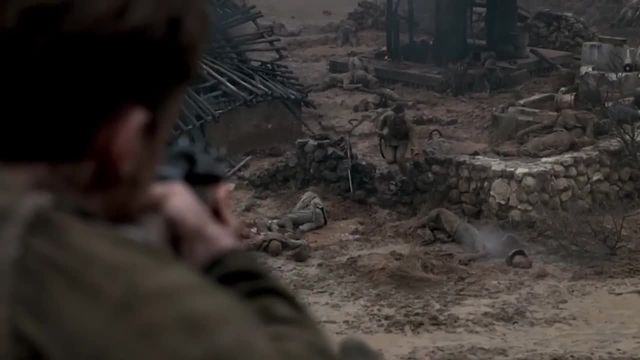 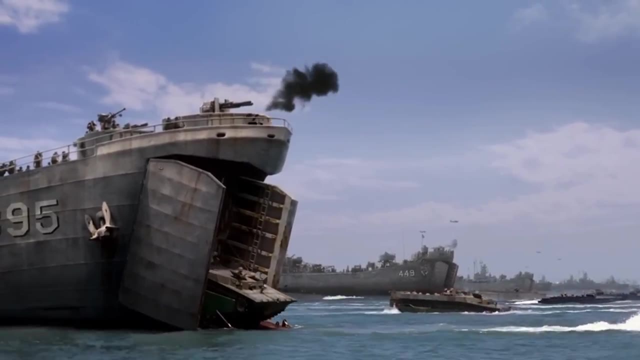 at the time of its release. In total, HBO spent around $217 million, According to co-executive producer Tony To. the commitment to realistically filming battle scenes was tremendous. Take the landing at Peleliu, for example, which took four days to film. 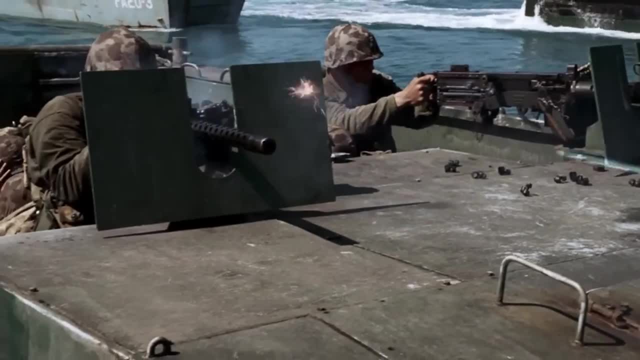 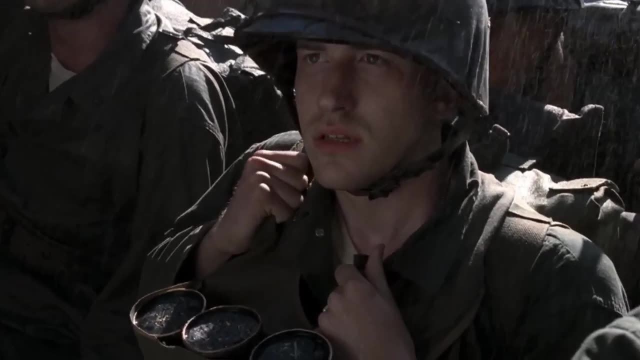 and came in under budget at around $5 million. The scene featured upwards of 300 actors, each of whom was clad in perfectly duplicated 1940s military uniforms that had been faithfully crafted on period. looms On top of the cost of working with a large cast. 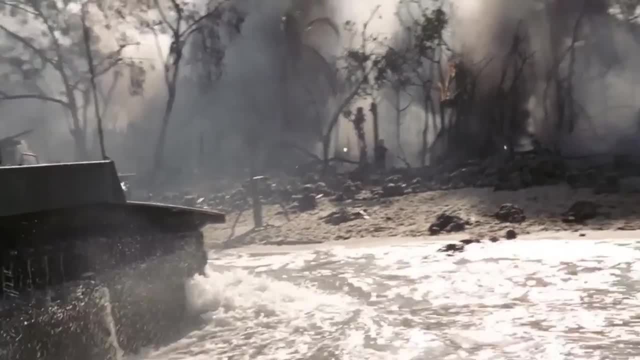 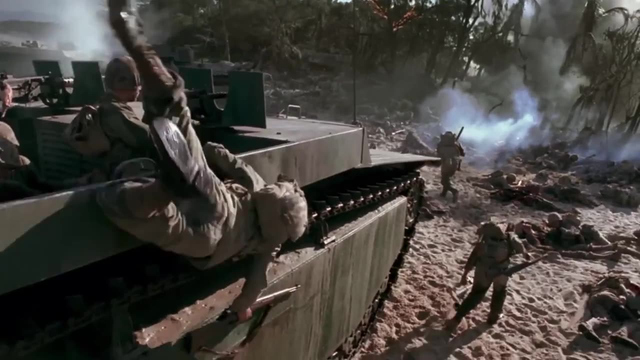 producers had to factor in pricey practical effects, props and pyrotechnics, With production cost coming in at around $270,000 per filming day. Fortunately, producers were able to cash in on rebates by filming in Australia, slashing the show's total costs by about $20 million. 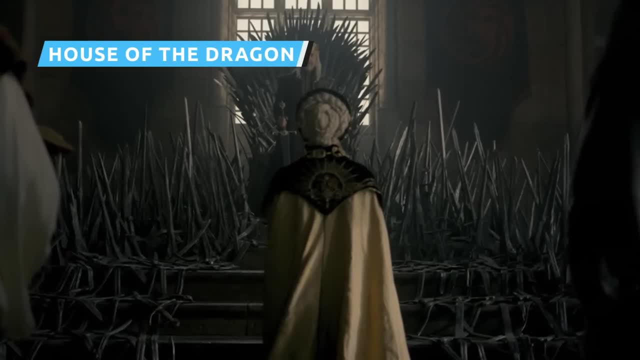 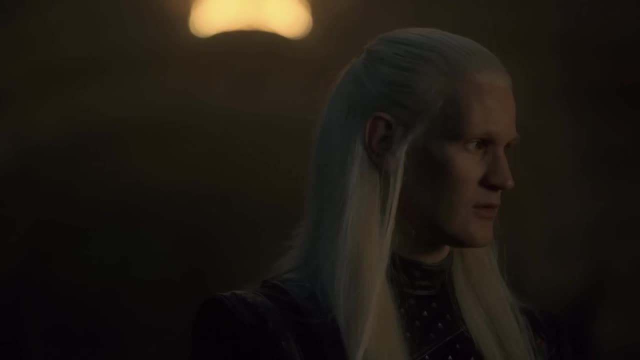 House of the Dragon is a prequel to HBO's absurdly successful fantasy drama series Game of Thrones, And, like Game of Thrones, House of the Dragon features an extra-large ensemble cast of several dozen actors, many of whom were already well-established names when filming began. The first season's budget was around $200,000, which comes out to about $20 million per episode. In comparison, the budget for the final season of Game of Thrones was around $15 million per episode. Fans of George RR Martin will be glad to know. 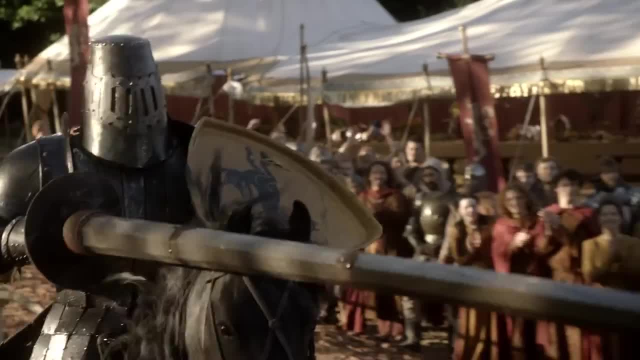 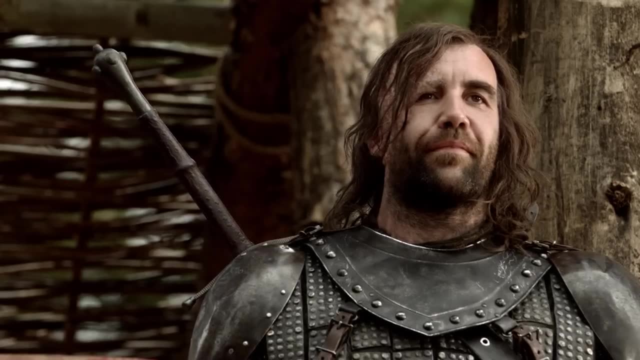 that Westeros is getting the treatment it deserves after cost-cutting led to some not-so-flattering moments in Game of Thrones, with Martin noting the first season's small-scale jousting tournament as a particular disappointment, Judging by the incomparable tawny in House of the Dragon. 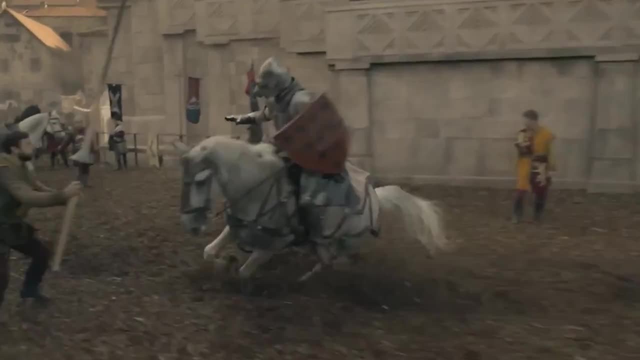 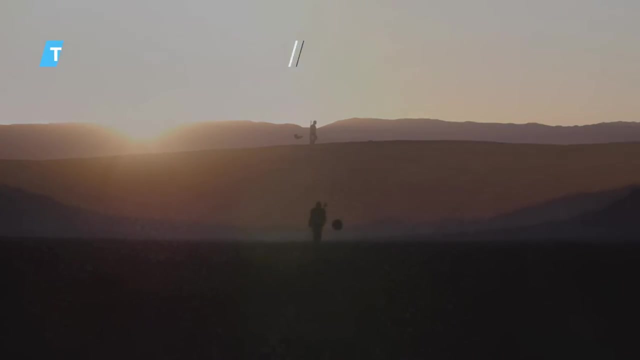 it's clear that the producers are going out of their way to avoid making the same mistake twice. The first of several live-action Star Wars shows to be released on Disney+, The Mandalorian, is a space western set a few years after Return of the Jedi.